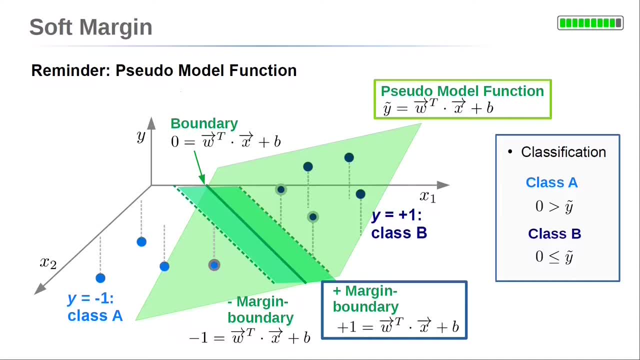 Further. for y, tilde equals plus one, we have the plus margin boundary which limits the margin to class B. For y, tilde equals minus one, we have the minus margin boundary which limits the margin with respect to class A. The margin is the space. 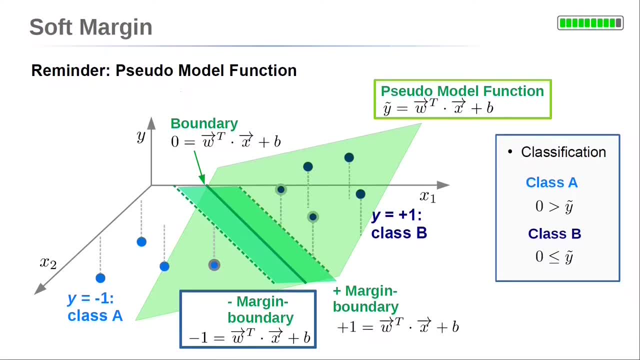 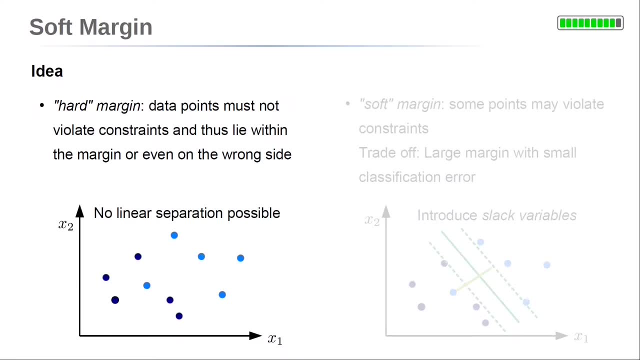 without any data points around the separating boundary. We used the support vector machine in the first culture of field genius at the management vector machine to classify two classes with a separating boundary. This boundary has a linear shape by its construction, But what if there are only a few data? 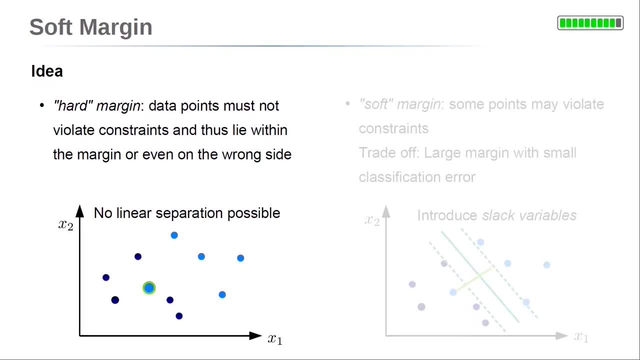 points which violate the linear separability of the classification problem. This situation is sketched on the lower left. Only a single light blue data point is among the dark blue dots. Without it we could apply directly the support vector machine. However, so far our margin does not allow. 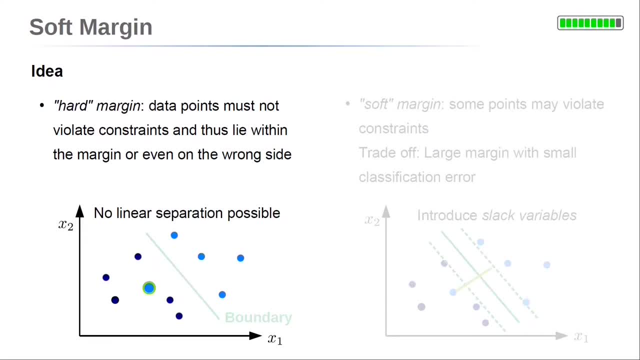 data points to be within the margin or on the wrong side of the separating boundary. This is called hard margin. We could use a variable transformation, but this seems not appropriate If only a few outliers violate the condition of linear separability. More appropriate is to weaken the hard margin constraints and allow a few data points to 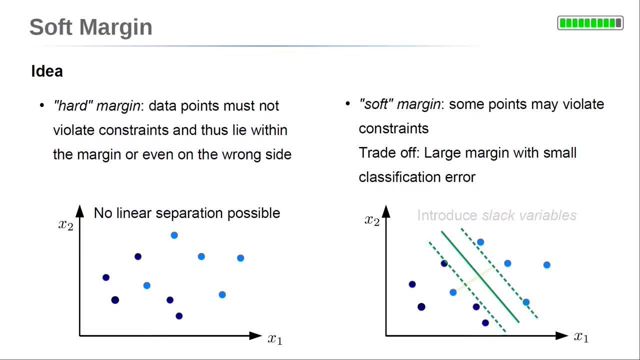 violate our strict separation conditions. This leads to the so-called soft margin, Thereby we have to find a trade-off between misclassified data and a maximal margin width. This procedure allows to apply the support vector machine to problems even if a few data points violate our constraints. To quantify the misclassification, the so-called slack. 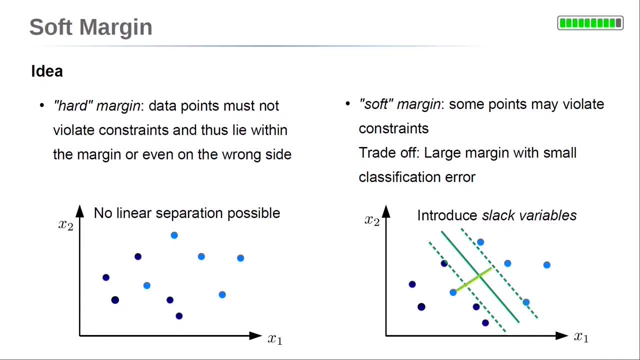 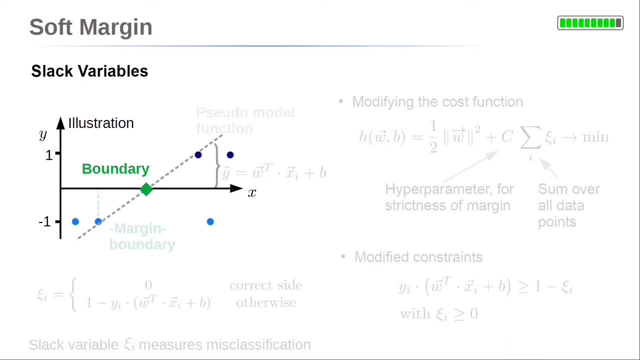 variables are introduced. Now let's consider a simple one-dimensional example where a single light blue data point is among the dark blue data points. Now let's consider a simple one-dimensional example where a single light blue data point is among the dark blue data points. 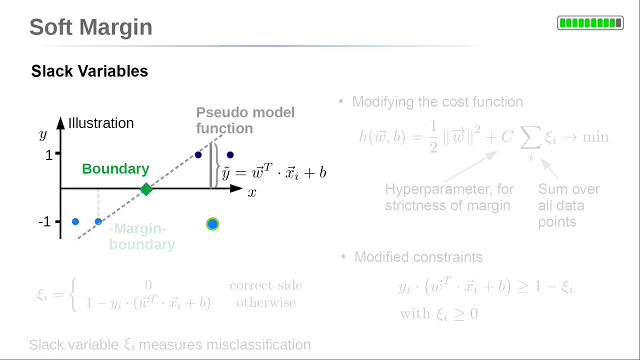 Our pseudo-model function y tilde has a certain value at the location of this data point. Our pseudo-model function y tilde has a certain value at the location of this data point. This value measures the misclassification with respect to the separating boundary. 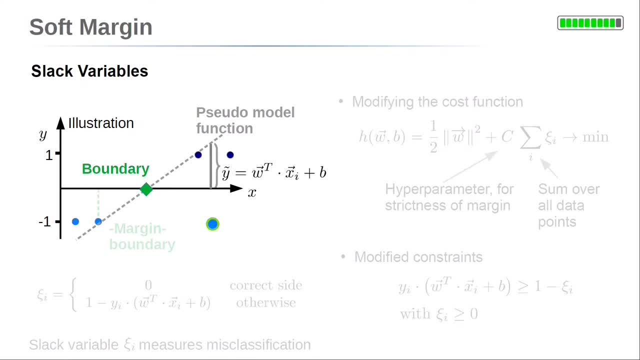 It is zero at the boundary and increases linearly outwards. However, our constraints state that the data points should not only be on the correct side, but also on the right side. However, our constraints state that the data points should not only be on the correct side. 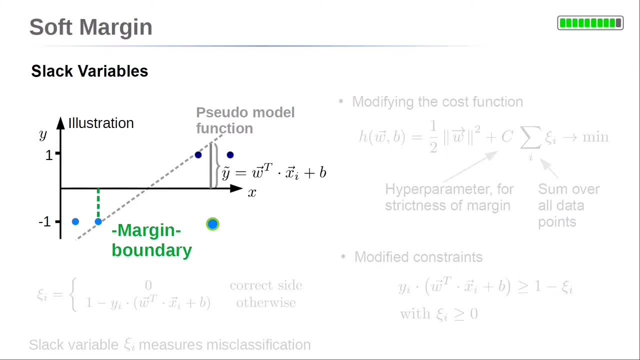 but also on the right side. For every point on the left-side of this separation, the data point should not be on the point on the left-side of this separation, nor of the right-side of this separation. The data points should be within the marking margin. 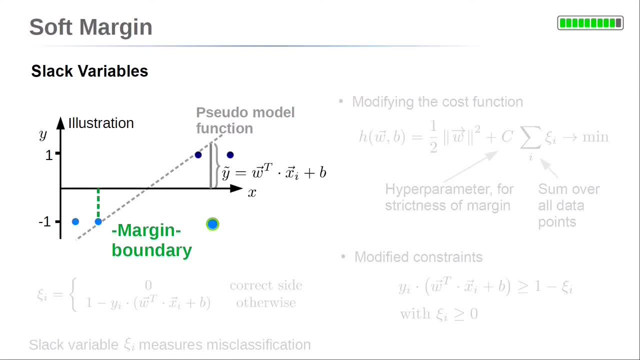 So it's a shape map. So we shift the value xů1 to the ここ x Ö1k. So we shift the value x Ö1k up to here Here: 1 plus y tilde. This expression measures the misclassification with respect to the minus. 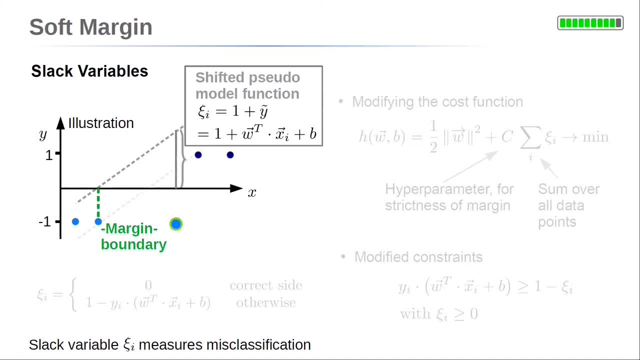 margin boundary, The contribution xi i decreases if the data point is closer to the minus margin boundary. At the minus margin boundary the value is zero. On the left side of the minus margin boundary the measure of misclassification should be zero. So we set xi i is equal to zero. 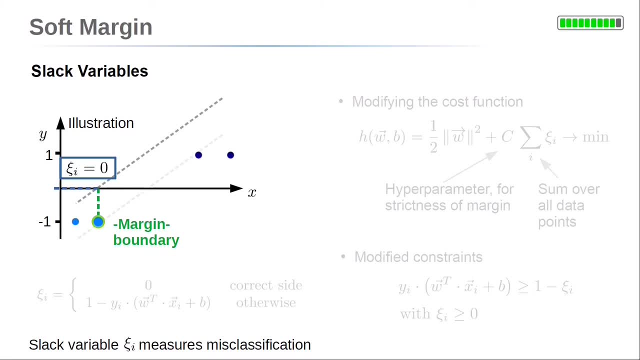 for all points on the left side of the boundary. In total we have xi i equals zero on the correct side of the margin boundary and xi i equals 1 plus y tilde. otherwise, So far we considered only misclassifications of the light blue data points of class A. 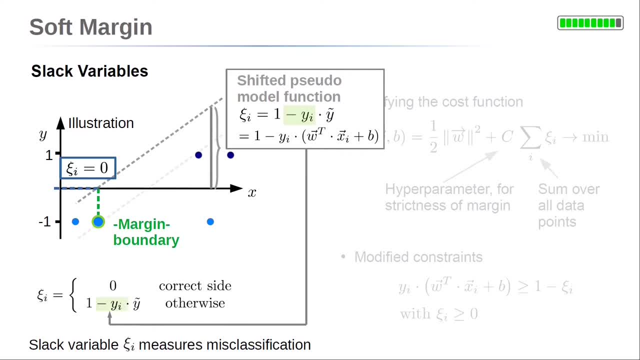 To incorporate class B as well. we write: instead of 1 plus y tilde, 1 minus y i times y tilde y i equals minus 1 for class A. These are the light blue data points. So this holds our previous considerations and we still have 1 plus y tilde for class A. 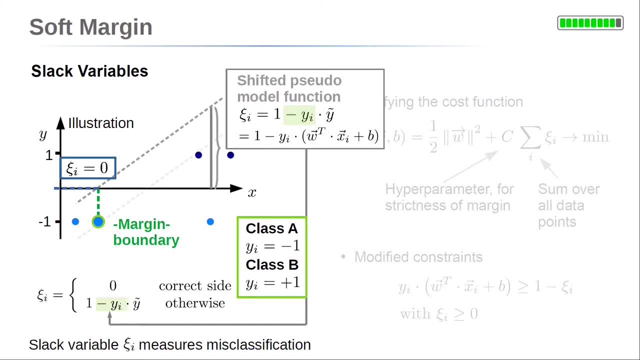 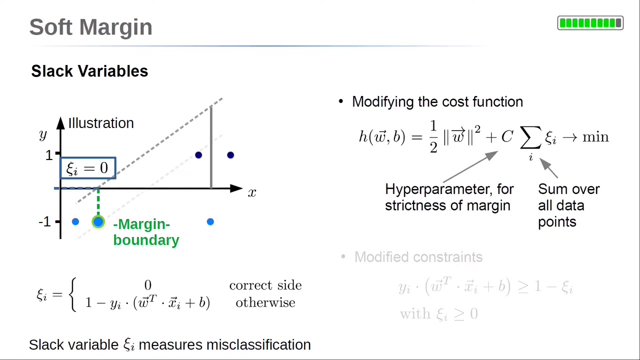 However, this more general expression also holds for class B. We can substitute the pseudo-model function y. tilde equals the parameter vector w, transposed times the vector of the input variables x plus the parameter b. The cost function is modified to include the slack variable into the model. 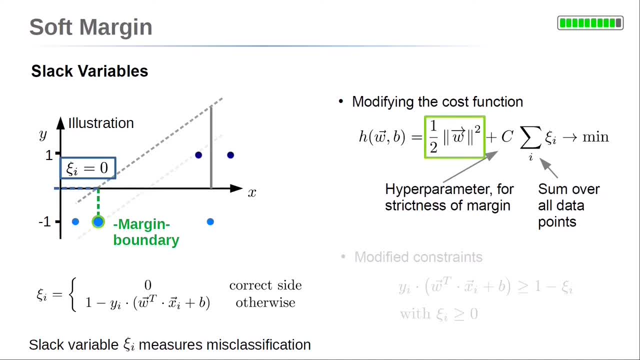 The first term, one half times. the parameter vector w squared still wants to maximize the margin width. The second contribution, c times the sum over all data points of the slack variable values, incorporates the amount of margin width. This works as a multiplication violation. 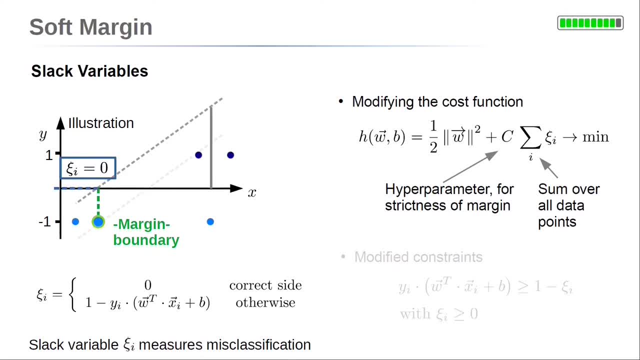 So minimizing the cost function needs to balance the maximization of the margin and at the same time not too much violation of the separation of the classes. The new hyperparameter c specifies this trade-off. Large values for the hyperparameter c lead to a hard margin. 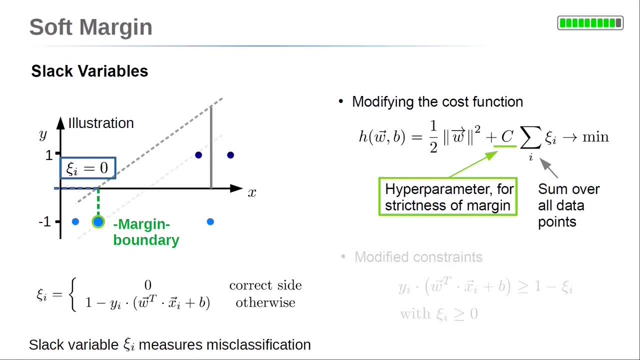 This is because of the large contribution of the hyperparameter c to the margin. solutions of the slack variables measuring the misclassification. Small non-vanishing values for C lead to a soft margin which allows for more violation of the margin. Now let's check our constraints: yi times the parameter vector w. transpose times the. 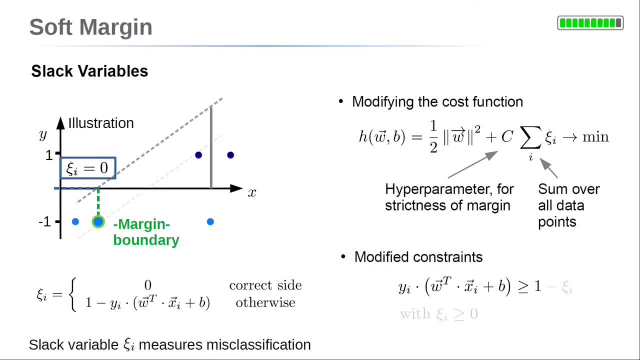 data vector xi plus b is greater than or equal to 1.. These constraints are modified to allow for violation. The slack variable for the corresponding data point is subtracted on the right side. When we take a look on our definition of the slack variable, we can see that the data point 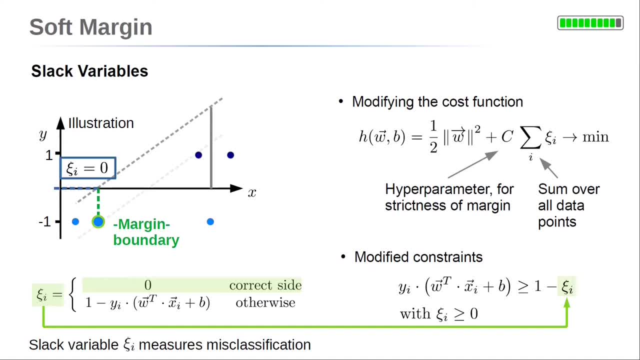 on the correct side still gives our original constraints. So for xi i equals 0, we have our original constraints. However, for a data point on the wrong side we can substitute xi i into the constraint inequality. The 1 cancels out and on both sides we have yi times the parameter vector w transpose.